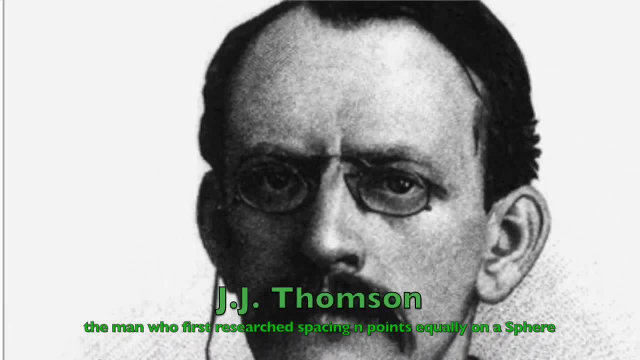 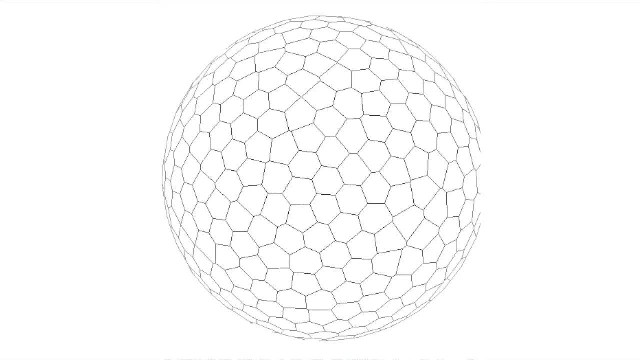 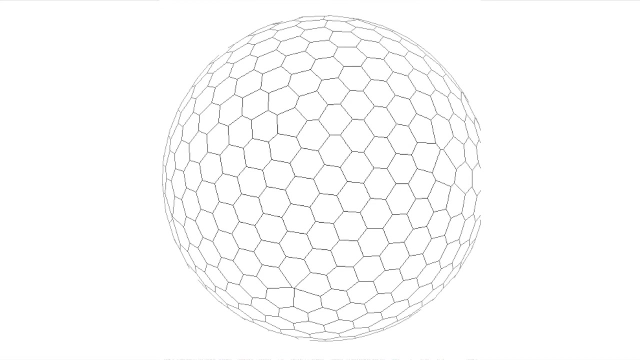 In the past, work has been done on creating algorithms to space any number of points equally on a sphere. The best methods use calculus and they work by having all of the points repel each other continuously until they reach an optimal configuration. The problem with these methods is that they are extremely slow and for large numbers of 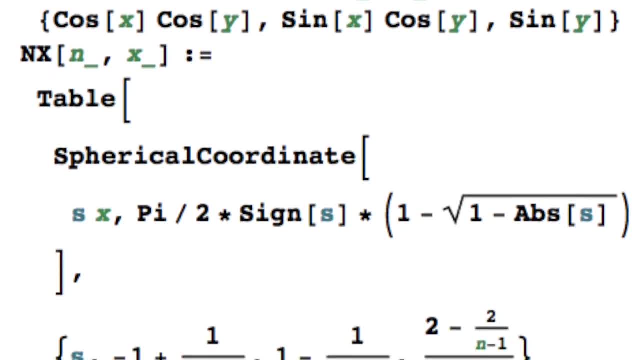 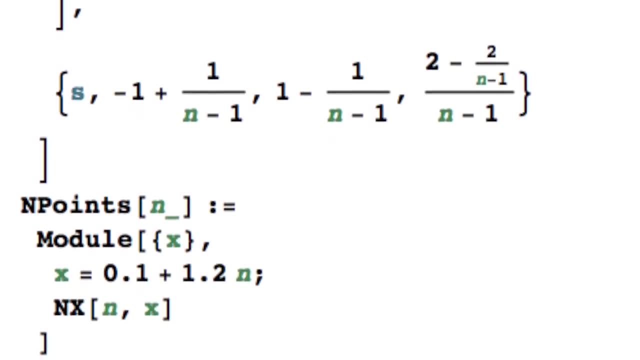 points. they take a long time. What I have created is an accurate algorithm that spaces n points equally on a sphere without using calculus, allowing it to work on large numbers of points efficiently. The first step in creating my algorithm was I used spherical coordinates to program a. 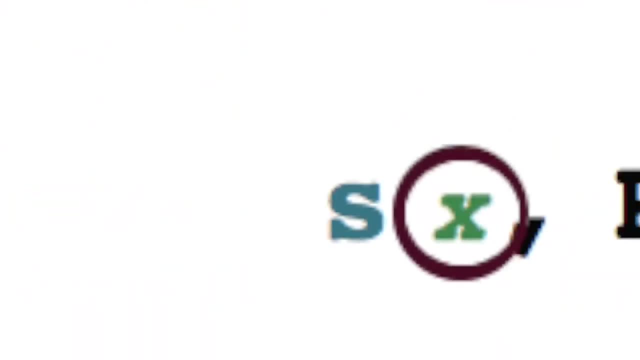 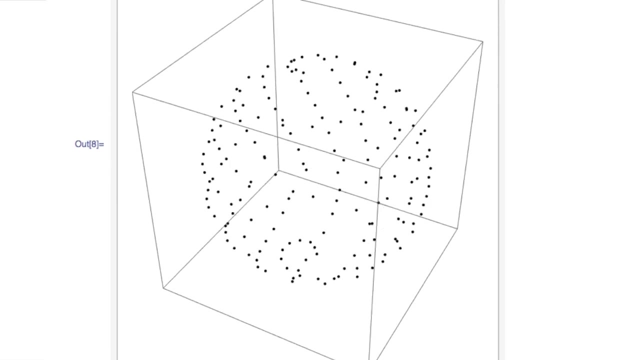 function that put a spiral around a sphere. I then added a new variable called x, which allowed me to manipulate the broadness of the spiral. As I changed the x, I found that some configurations of the points appeared to be much better than others. 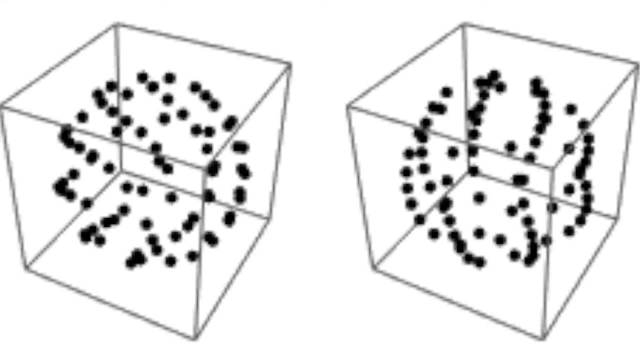 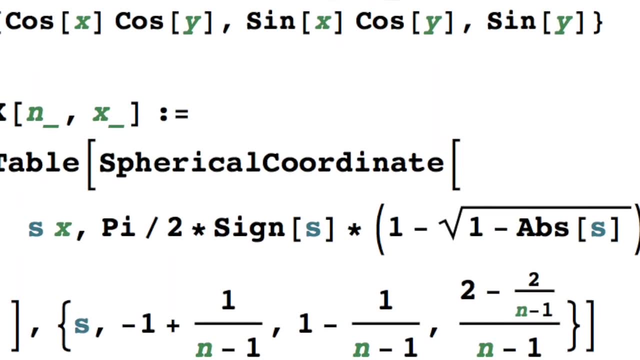 At this point. I went out and found many optimal n-x pairs. When I closely observed the configurations of points, I realized that there was clumping at the poles. I fixed this by having the spiral stop just before they reached the poles, allowing me to raise the accuracy of the function. 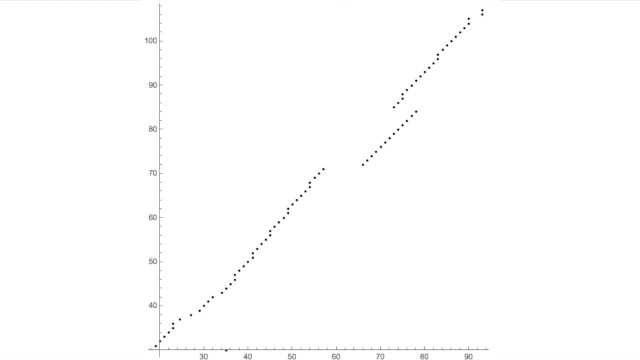 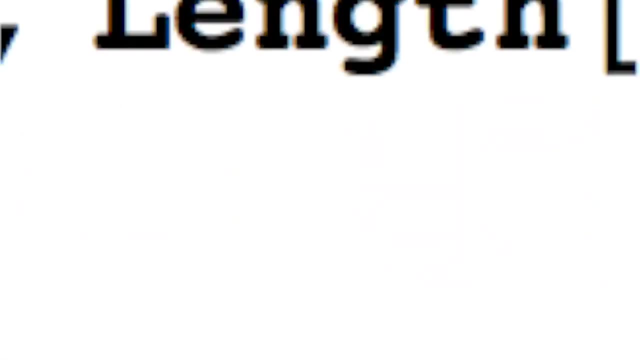 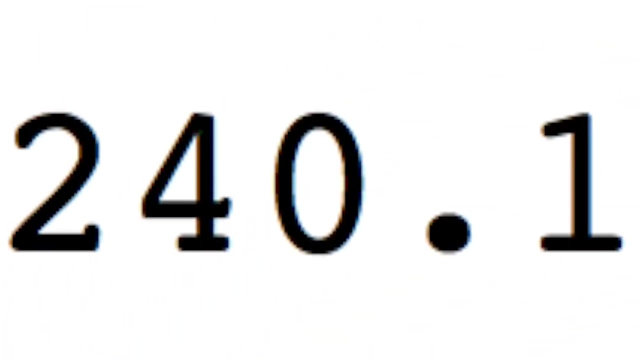 After this, I then plotted the pairs and noticed that they appeared to be part of the linear function. Using this knowledge, I realized that I had to find the linear function that provided an x for every n. I did this by developing a few accuracy functions, and I then used them to find that the optimal x for 200 was 240.1.. 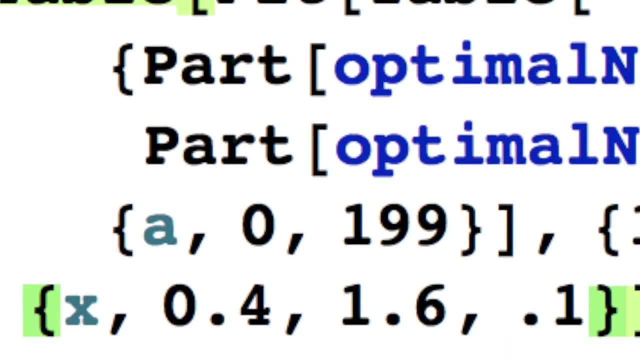 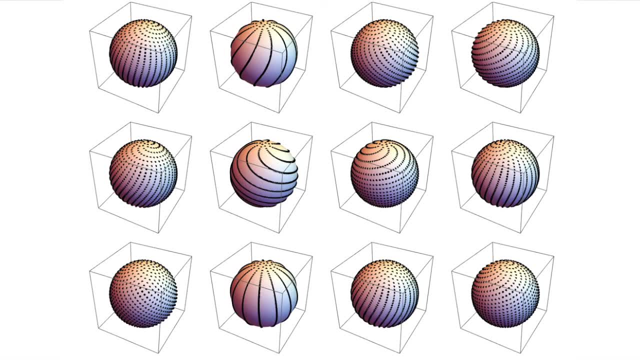 Seeing that the linear function from before had a slope of around 1,, I tried a bunch of different slopes near that for my function. I then continually narrowed it down until I found many different functions that were almost indistinguishable. I then plotted these optimal functions' accuracies. 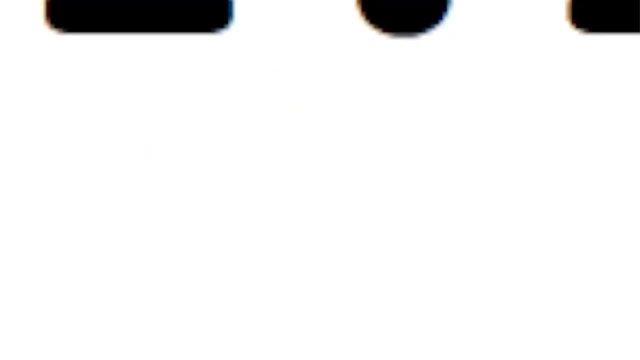 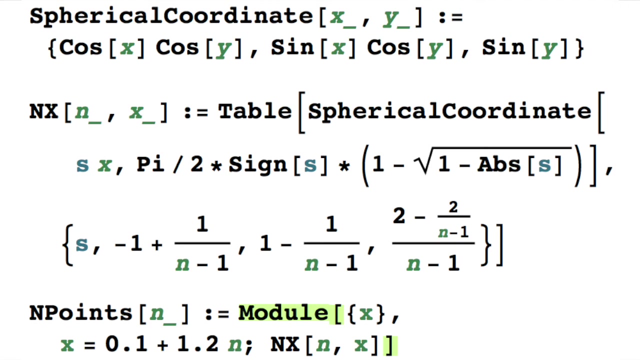 The one that stayed the highest for the longest was the best. This function was 0.1 plus 1.2n. I then put 0.1 plus 1.2n in as the x in the function, and the results were great. 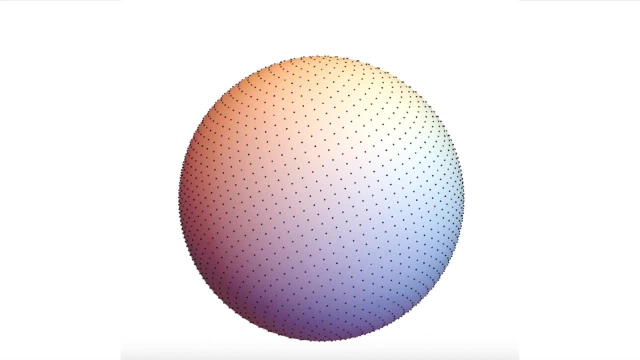 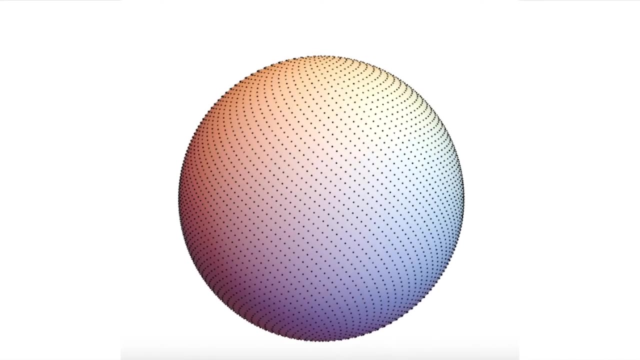 As you can see here, the function worked for any number of points quickly. When analyzed, the accuracy of the function ranged from around 70% to 86% and was incredibly fast, even as I got to numbers of points as large as 50,000,.